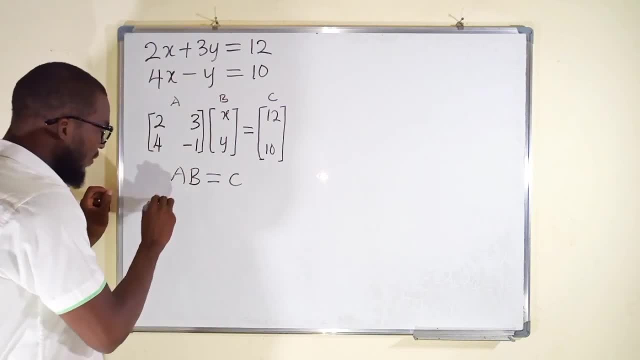 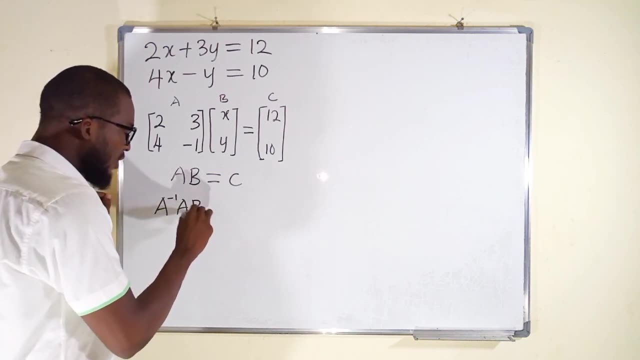 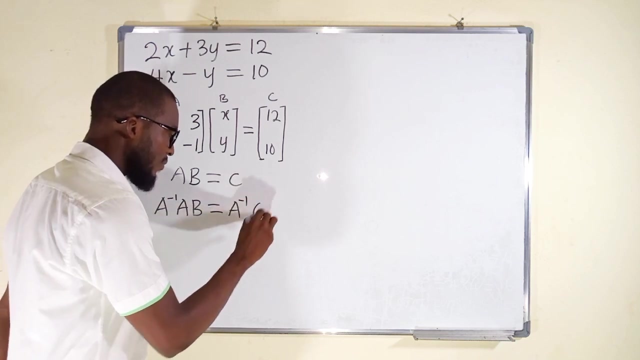 inverse of matrix A, because inverse of a matrix multiplied by the original matrix is nothing but an identity, An identity multiplying any matrix will not change the matrix, So we are going to multiply both sides by this A inverse. This will eliminate this entirely, leaving B And B. 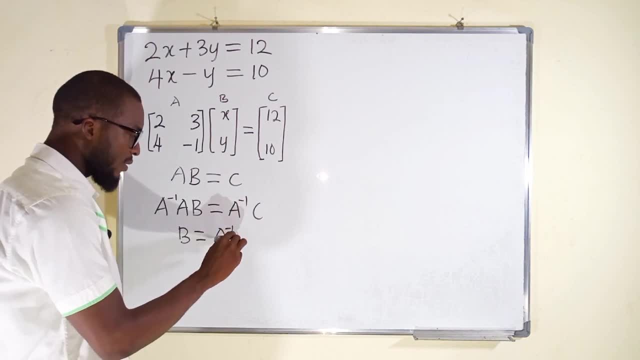 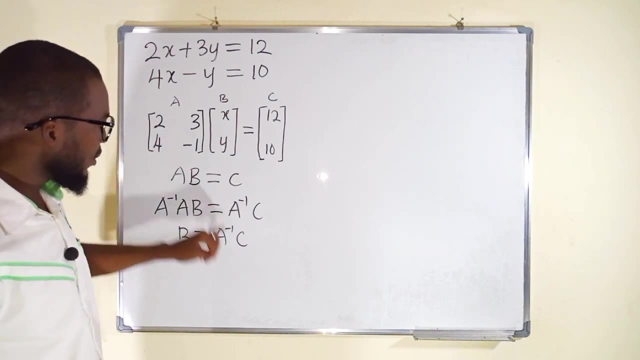 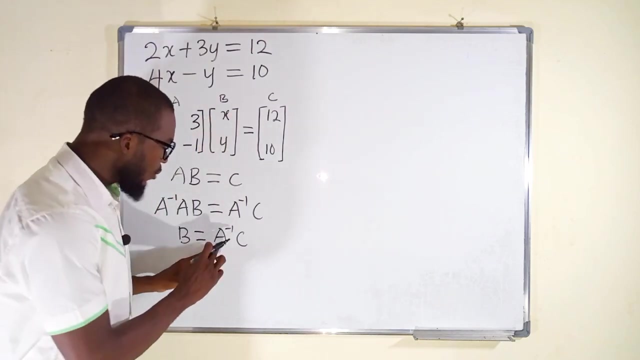 is equal to A inverse multiplied by C. What does this mean? It means that if we find the inverse of this matrix and multiply it with the constant, we are going to obtain the value of B, which represents our unknown variables. So how do we find inverse of a? 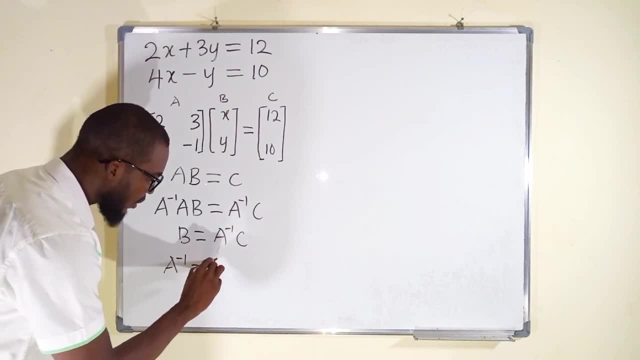 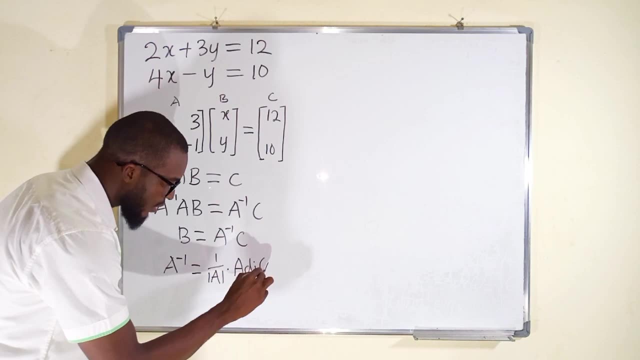 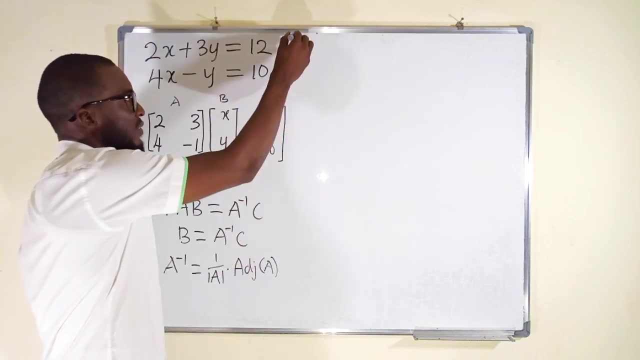 matrix. This A inverse is nothing but 1 over the determinant of that matrix multiplied by the adjoint of the same matrix, A. So we are going to find the determinant of this matrix as well as the ad join of the same matrix. Let me start by finding the determinant, The determinant which is: 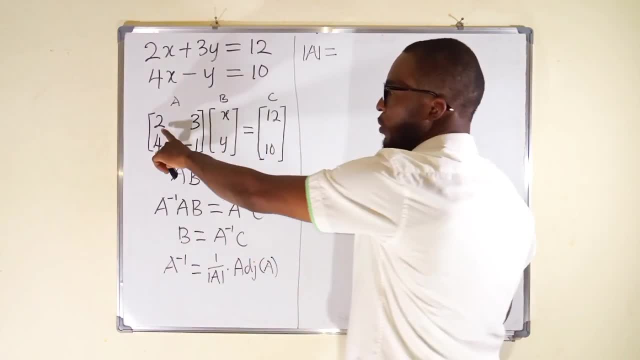 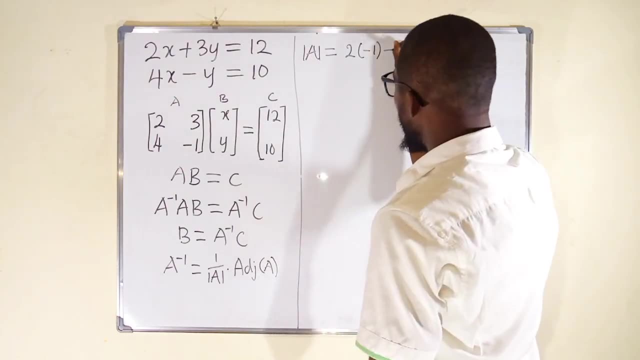 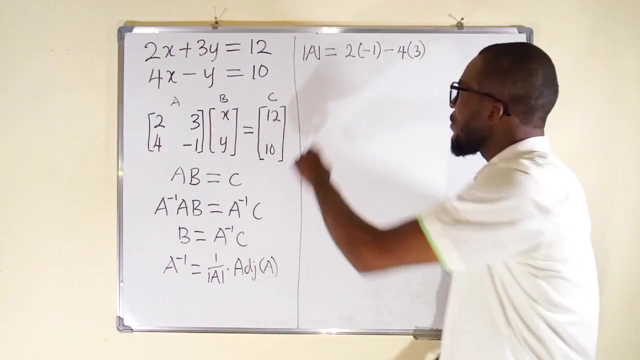 denoted by This is equal to B. You take 2 and you multiply by the legion diagonals, Then you subtract. You take the other diagonal. We have 4 and we multiply it by 3. You can see that 2 multiplied by is weil. 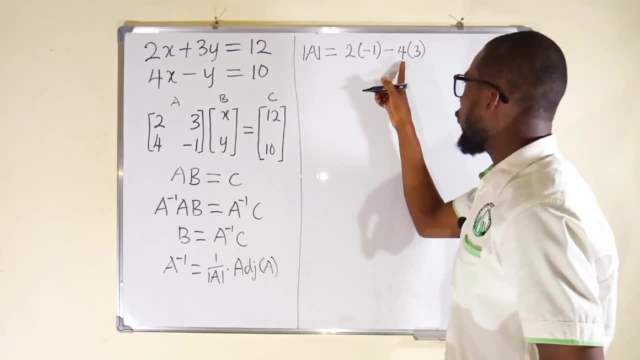 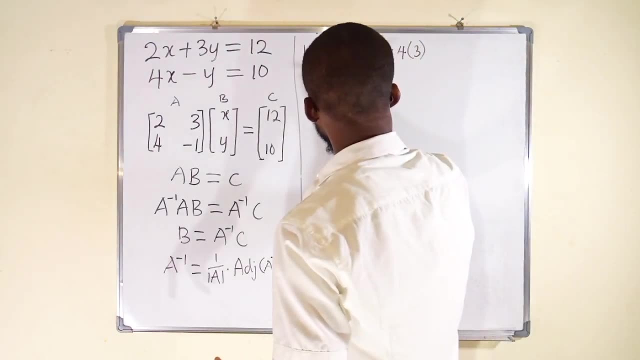 podium aconteceu. 006- 007-0-1responsible. negative 2 is negative 2, as you would expect, and negative 4 multiplied by 3 is negative 12. negative 2. negative 12 is negative 14. this means that the determinant of this matrix is nothing. 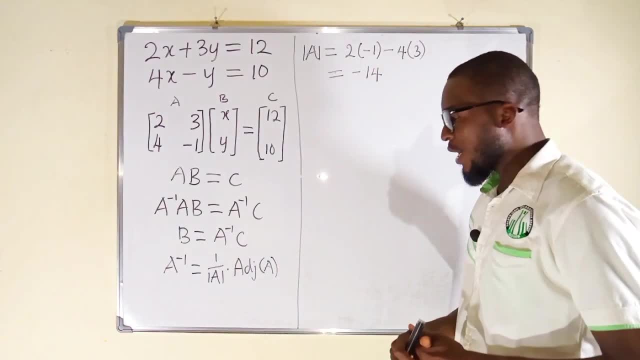 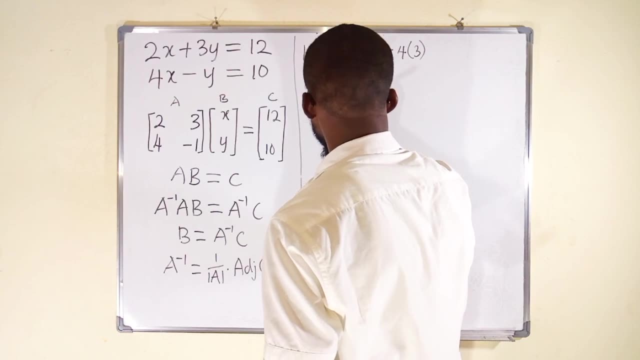 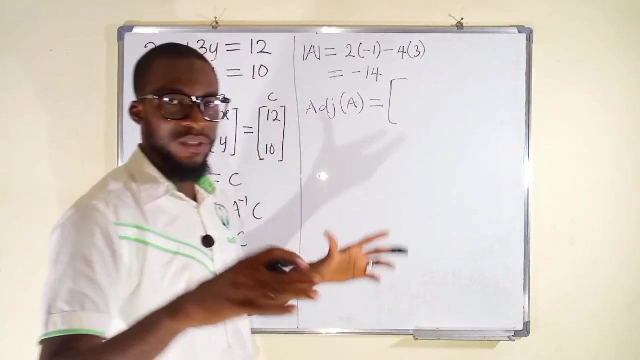 but negative 14. now let us go ahead and find the adjoint of this matrix. the adjoint of this matrix. I'll follow a shortcut, because I have shown you how to find the adjoint of a matrix in our previous lesson. so for 2 by 2, we are. 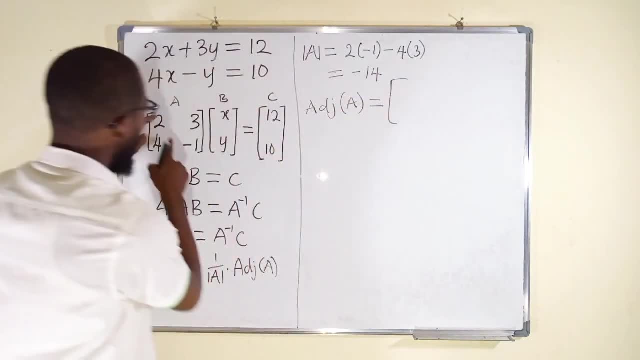 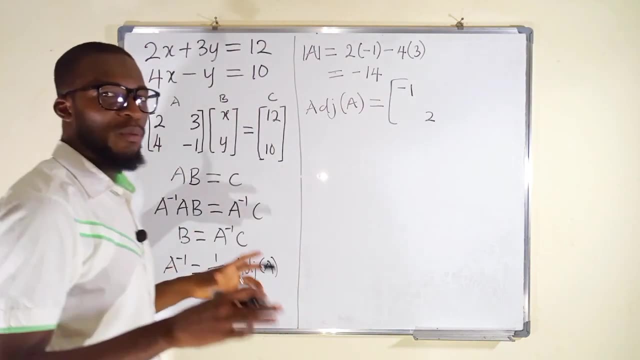 just going to interchange the leading diagonals. we have 2 and negative 1, so I will start by writing negative 1, then 2, then the other diagonals. I am going to multiply them by negative 1. we have for this: we have negative 4 and for this we: 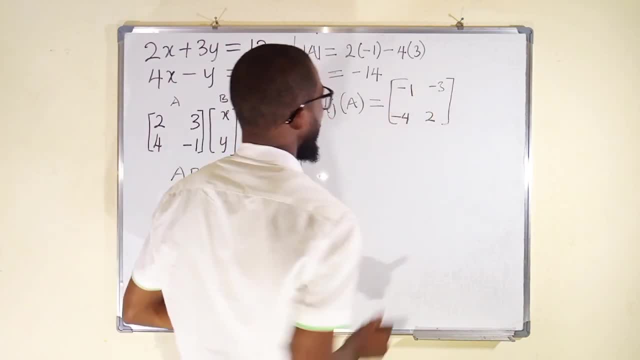 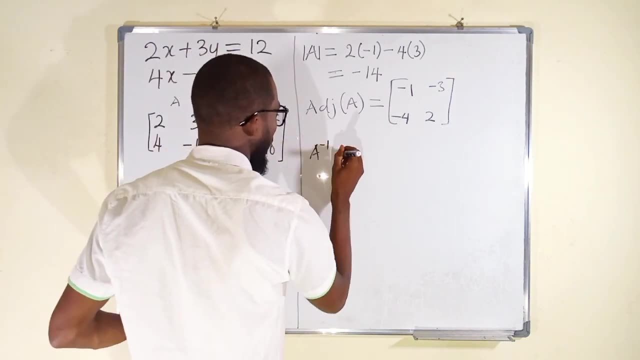 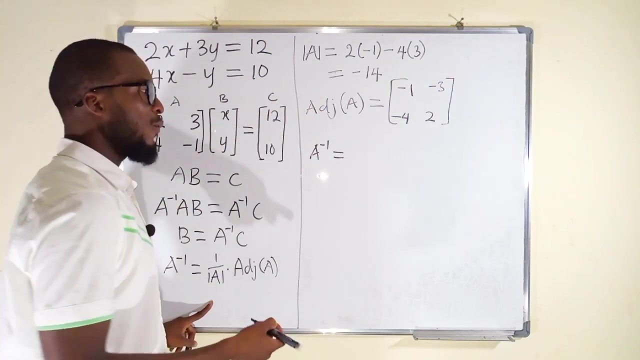 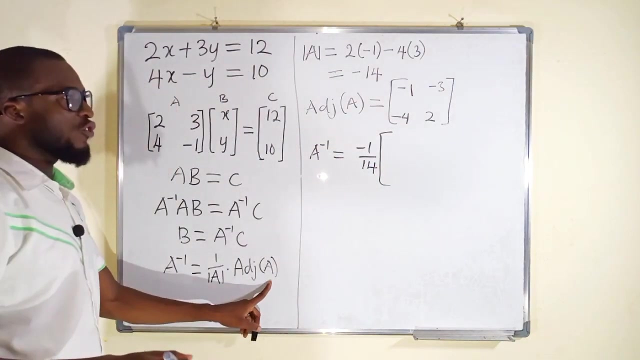 have negative 3. this is the adjoint of this matrix. then, for a inverse, which is the same thing as 1 over the determinant, the determinant is negative 14. 1 over the negative 14 is something as negative 1 over 14 multiplied by the adjoint, and this adjoint is negative 1, negative 4. 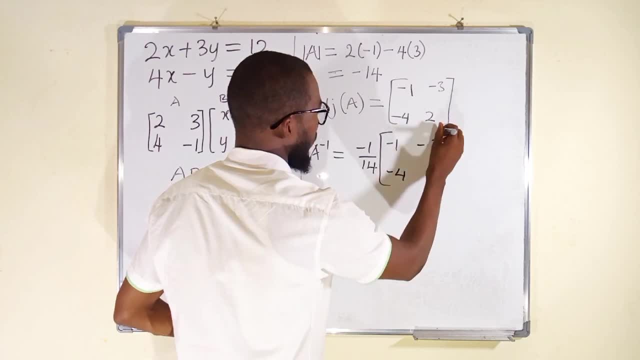 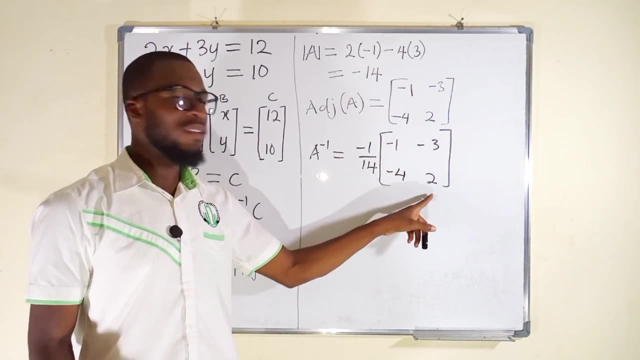 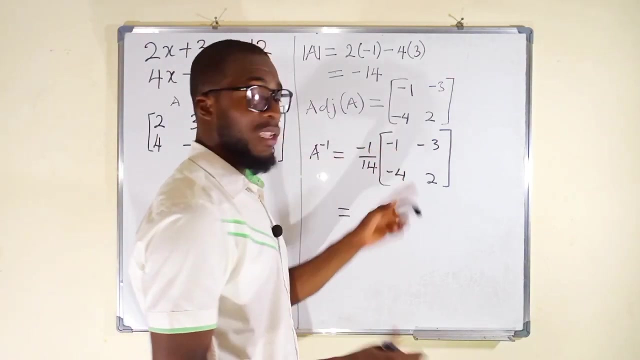 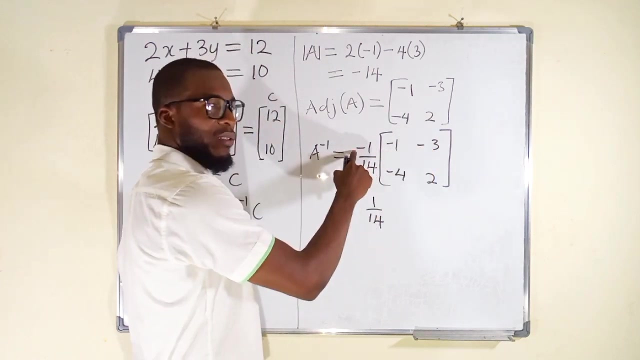 negative, 3 and 2. so this is going to serve as a scalar. and then each and every entry in this matrix and this equals, this time this will just change the sign negative, negative is positive, so we have 1 over 14 here. this other one will also cancel this negative sign to positive. we have. 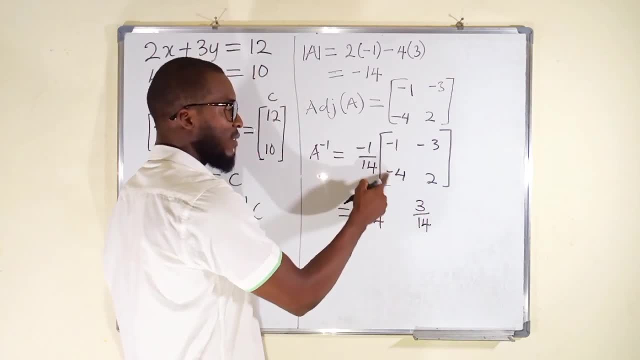 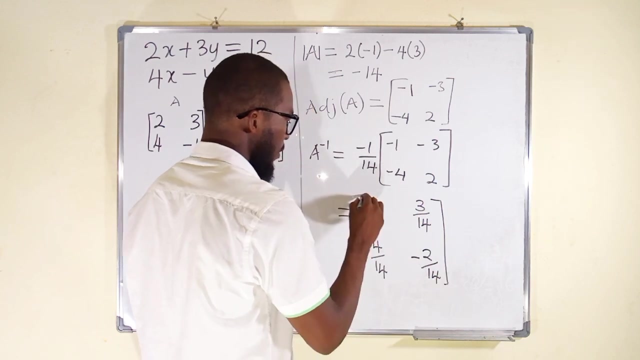 3 over 14 coming down here, this negative will changes. we have 4 over 14 and the last one, this is positive, this is negative. it will cancel this negative and remain negative. 2 over 14, and hence this matrix is said to be the inverse of. 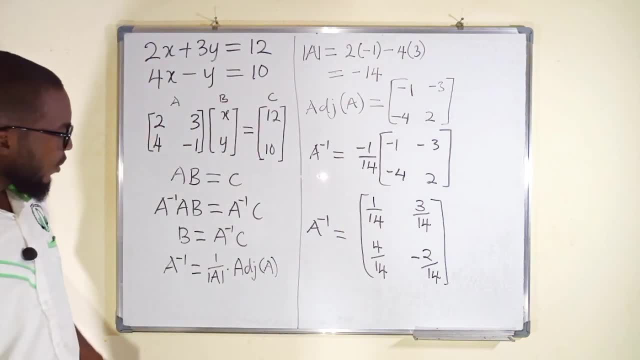 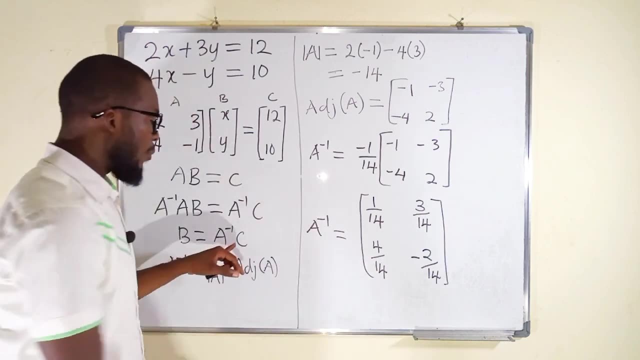 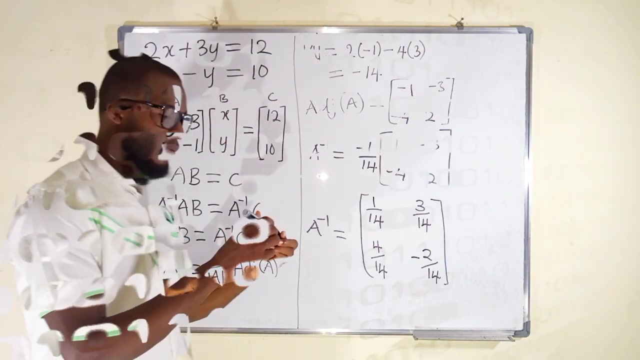 matrix a: okay, let's continue to find B, which is the required solution. we are going to take a inverse, which is this: multiply it by the constant, which is this: 12 and 10. so let me use this space for that. So, A inverse multiply by C, we. 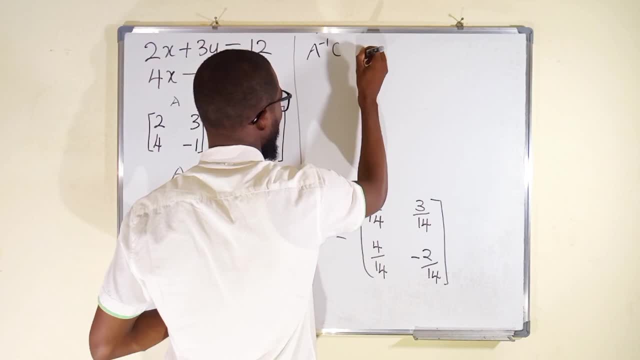 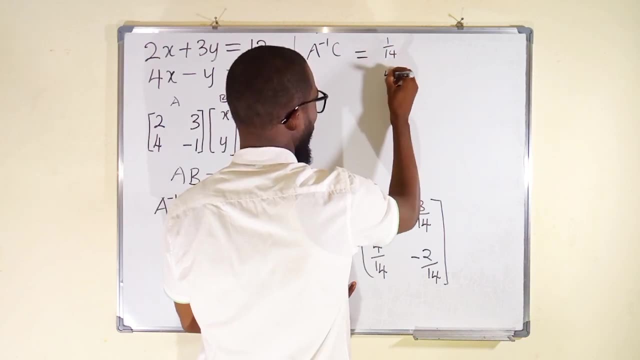 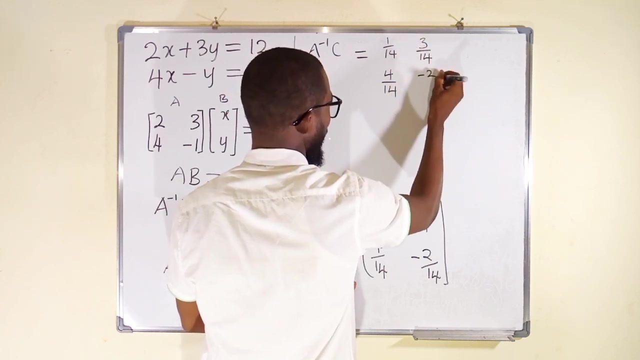 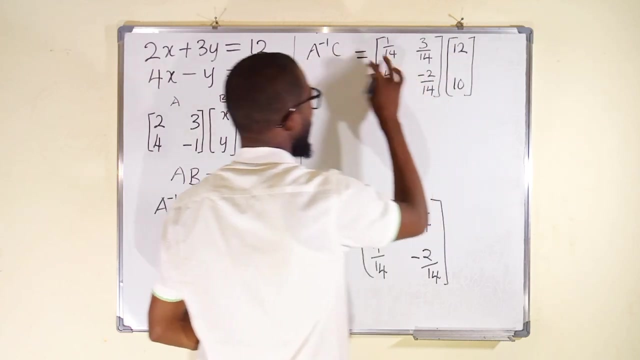 have A inverse multiply by C. this will give us- this is a inverse which is 1 over 14, 4 over 14,, 3 over 14 and, lastly, negative, 2 over 14. this is our A inverse multiply by C of us. then, for the constant, we have them as 12 and 10. we have 12. we have 10. 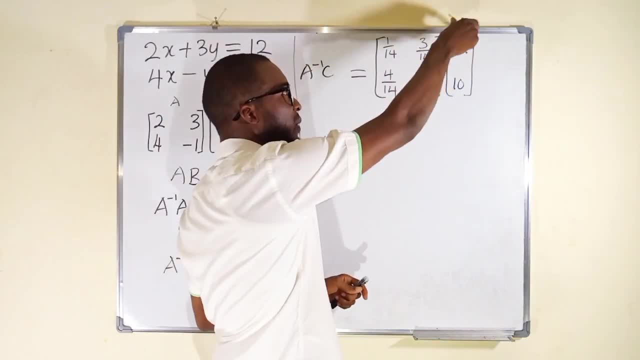 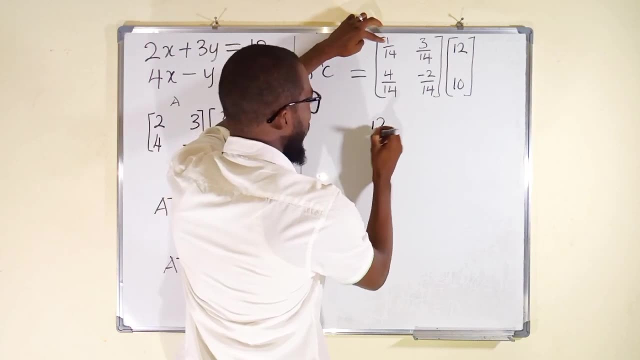 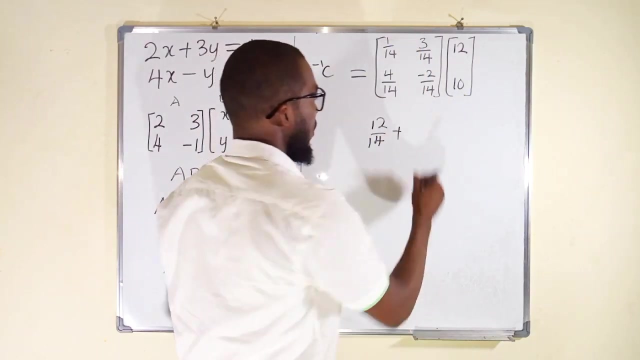 so we are going to take first row here and multiply it with this first column this time, this is going to make it 12 over 14. plus you take this, you multiply by this, 10 times 30 is 30. we have 30 over 14. then you take the second row. 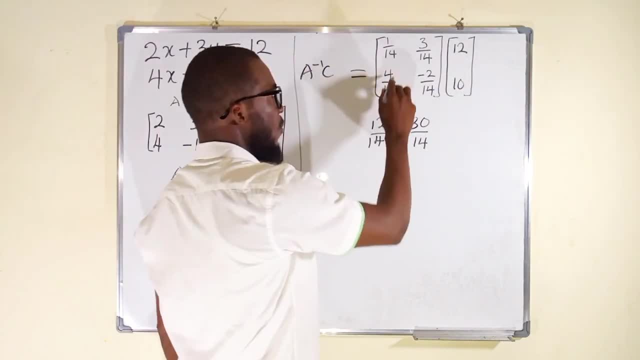 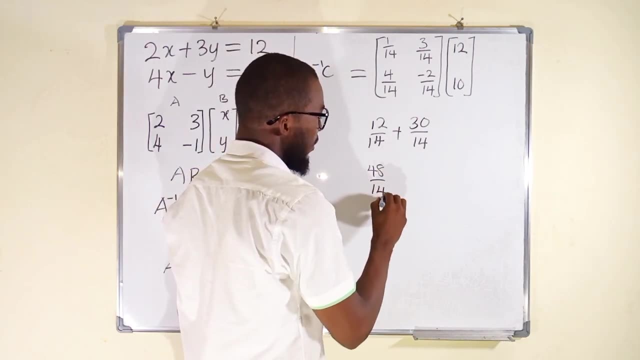 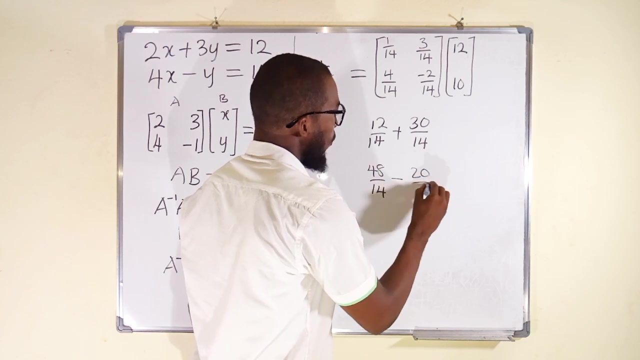 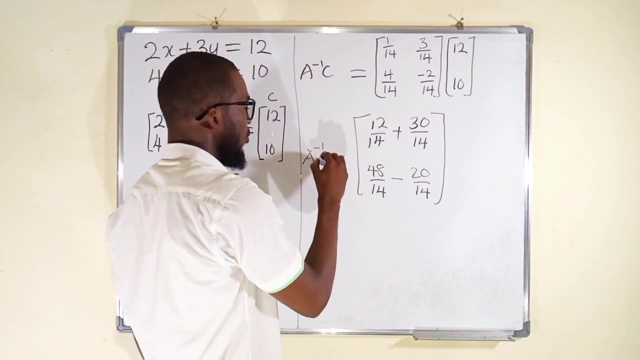 multiplied with that first column, 4 over 14 times 12 is going to make it 48 over 14. uh, negative 2 over 14 times 10 is negative 20 over 14.. remember, this is a inverse multiplied by c. let us further simplify this: plus this is going to make 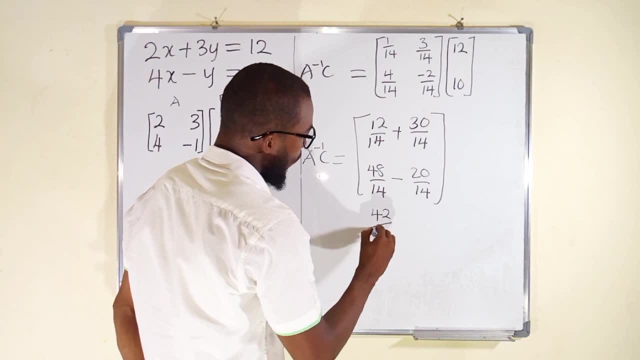 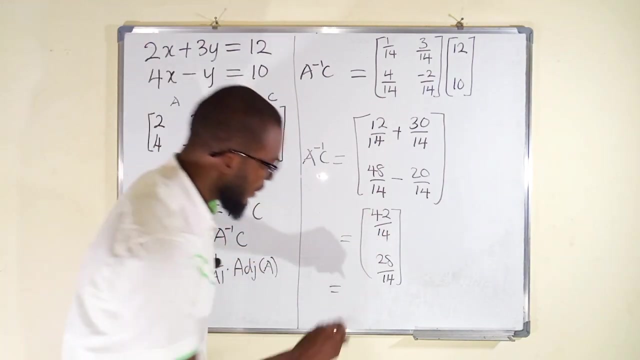 it um 42 over 14. this minus this is going to make it 28 over 14 down. and lastly, 42 over 14 is 3.. 28 over 14 is 2. drawn, this is a inverse multiplied by c. but what is this? a inverse multiplied by c? 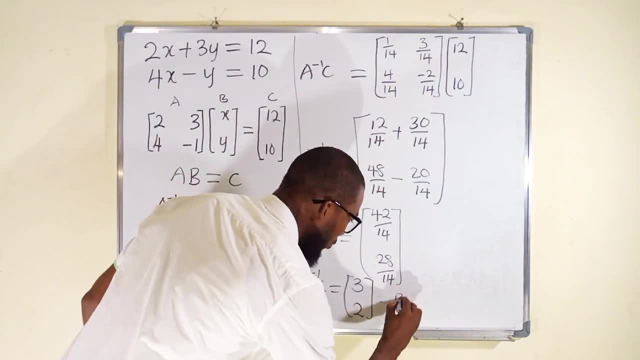 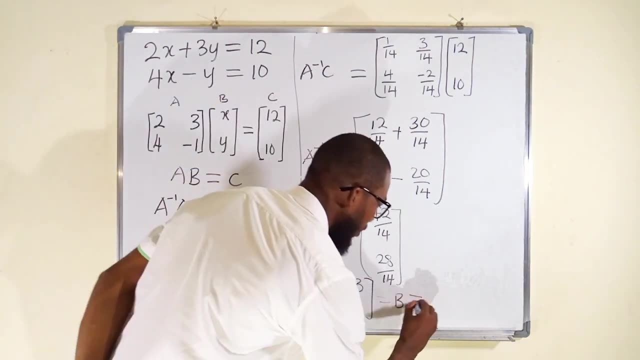 remember, it's the same thing as b. this is equal to b. and what is b? huh, we learned that b is the same thing as x and y, a matrix of x and y, x, x, x, x, x and y, y, and you'll see in. follow me to see how the matrix is like. thisibile estas capa. this is буквally 2. Here we have E1, total, same dot B as 1, plus H, x, Hcos B. This Is equals to b. And what is B? we learned that b is the same thing as x and y. when property x is equal to B, The formula is: 2 times C, 5 times A. this is equivalent to B. Again, no problems with this. persuasive things about where we have come up. so, while it was scrolling down a level at the tutorial, 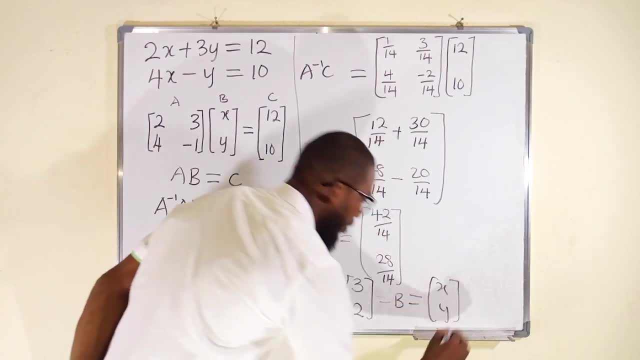 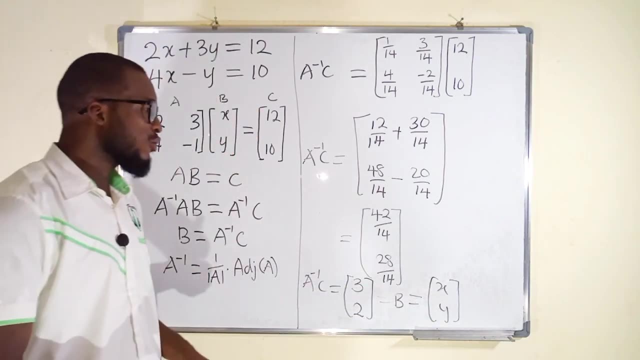 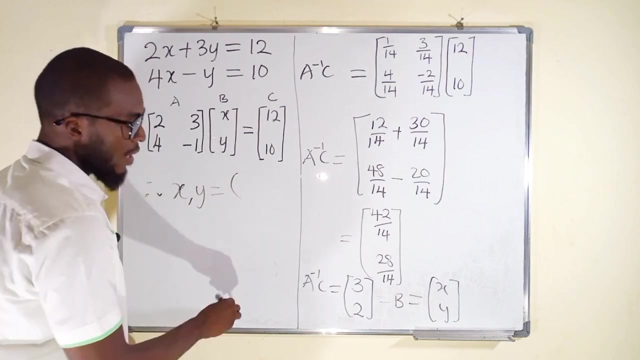 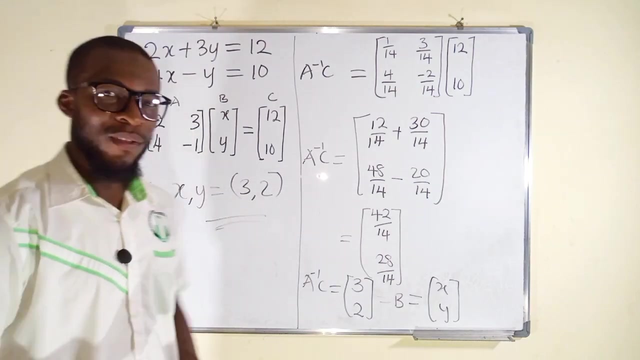 and y, x and y. so by relating this together, you can see that x is equal to 3 and y is equal to 2. so now let us conclude. therefore, x and y, the values of x and y are 3 and 2 respectively, and this is all i have for you today. thank you for watching. do have a nice day.